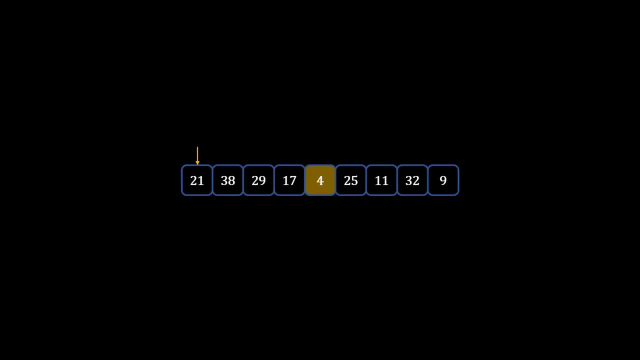 list, find a minimum number, which is 4 in this case, then you swap with the first element. After that, the first element is sorted. So now you move on to the second element. You want to find the candidate for the second position. And what is that element? Well, it is the second minimum element, or rather, 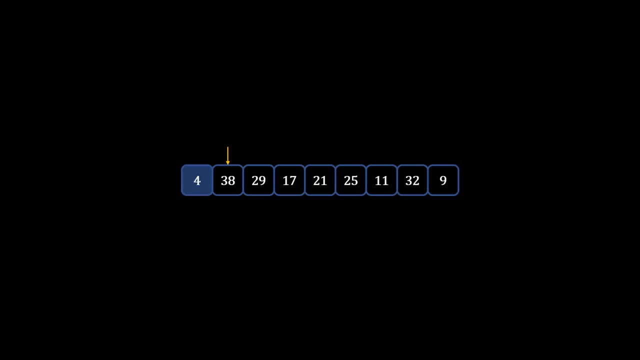 it is a minimum element in the unsorted array. So anything that starts with 38 onwards is unsorted and the left-hand side, which is 4, is sorted array. So in the unsorted array the minimum element is 9.. So you swap this one. 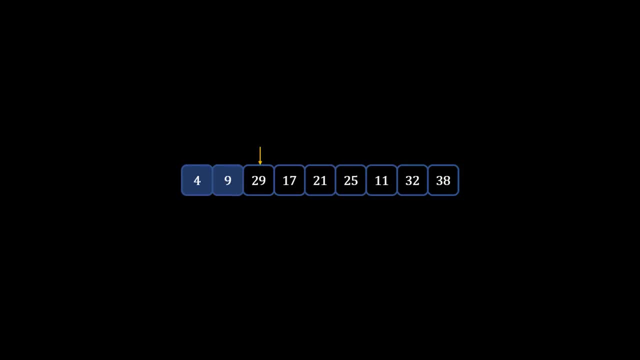 So you swap this one, So you swap this one with 9, and then you move on to the next element. If you keep on repeating this process, the entire list will be sorted. So this technique is very, very simple. Essentially, at every stage you have 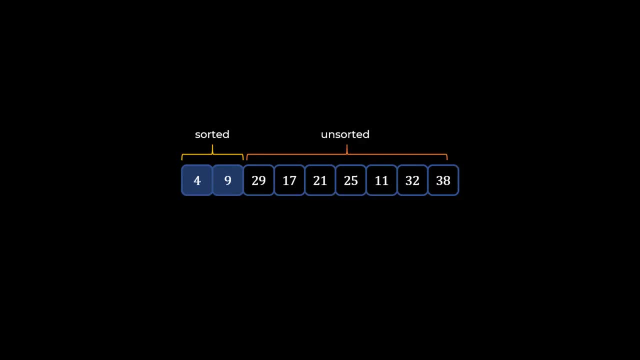 a sorted array and unsorted array. On the left-hand side you have sorted array and what you're doing in each iteration is: from unsorted array, find a minimum element, put it at the first position and move on. The local complexity of this is order of n square, Because you are already doing. 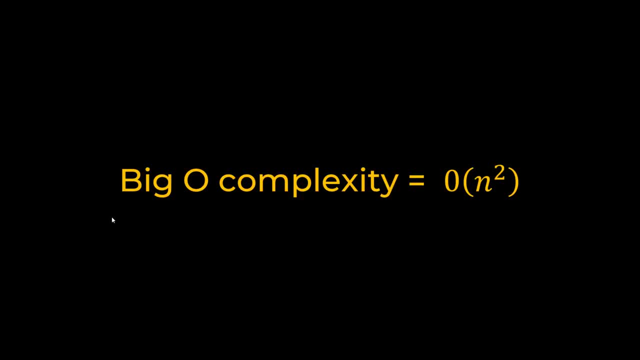 two of these for loop in your program, so it's not very efficient, But in certain cases it could be useful, especially when you have an extra space, And this is a very, very simple technique. When we write python code, you will see how easy the code is for this algorithm. 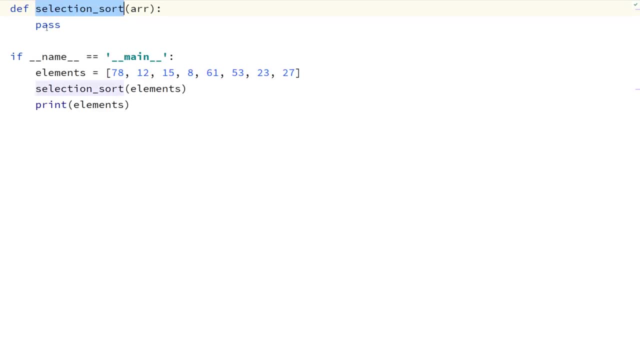 Let's write Python code now. I have an empty selection sort function on the basic running class and I am going to write code for that. The first thing we need to do is we need to write a code. find a minimum element from any list. how do you do that? well, let me just write a function which: 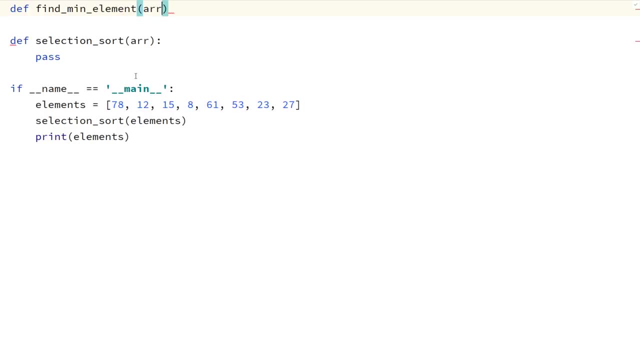 can find a minimum element. okay, so find a minimum element from an array. how do you find it? well, you can simply run a for loop for I in range, and just for simplicity. you know, I'll just remove this matter for now and I'll just say: okay, I want to just find a minimum element. you know, and I. 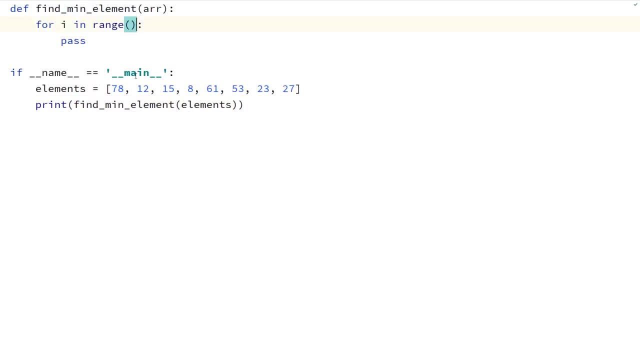 will just print it. so here you go through all the elements and then you define a minimum element. to be some minimum, let's say your list contains only positive numbers, the minimum number could be minus one. and then you will say: if array of I is, or rather actually for minimum, you need to initialize this to a very, very big number. okay, 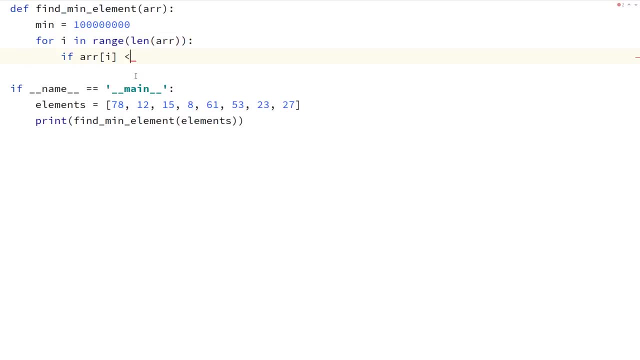 ideally it will be the max end, but I'm just for simplicity. I'm just initializing it to this number and if array of I is less than minimum, then minimum is equal to array of I and when you return minimum it gives you a minimum element. so let's run it really quickly. see eight. eight is the. 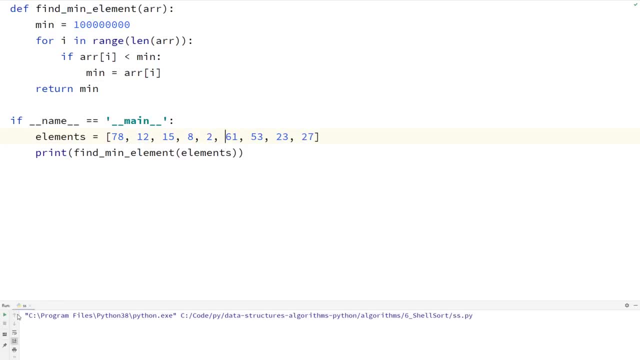 minimum element. if I have two here, it will put in two. now let's go back to our original function, which is selection short. so here let me just close this thing. I need to run two for loops, so the first for loop will give you an anchor. okay, so here for I in. so I just 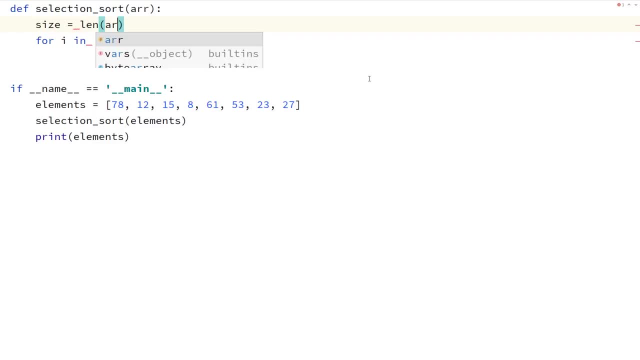 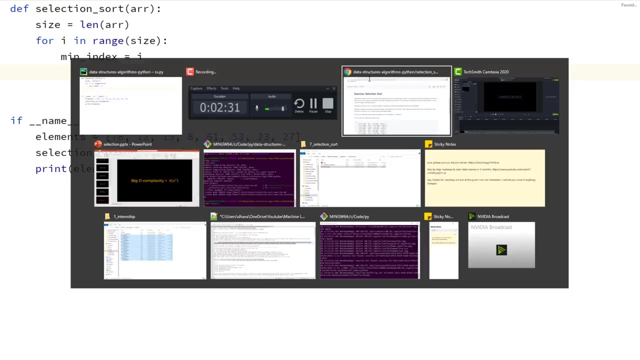 initialize the size into the size variable and you will say for I, in range size, okay, you go till size and do something. well, what do you do so here? first, you define the minimum index. so minimum index is your I. okay, if you look at our presentation, that minimum index is this thing. you know the. 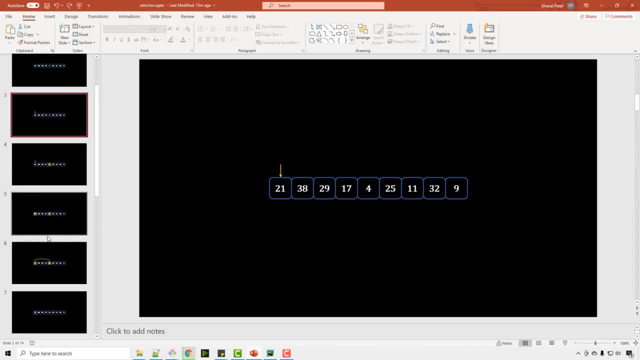 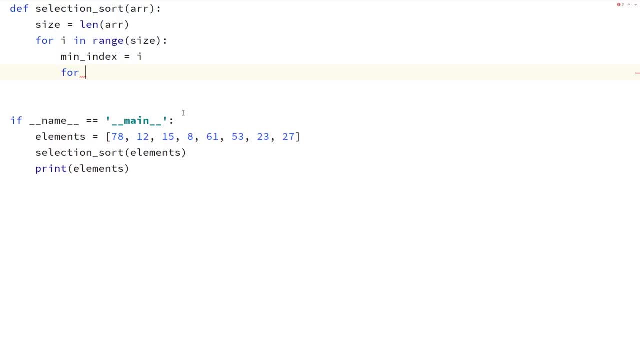 yellow pointer. so initially it will be zero, then in the next iteration it will be one, and so on. and in the second loop where you will say for J in range, something, okay, so J in range, mid index, you start with mid index plus one, go all the way till size, do something. so this loop is for this thing. so here: 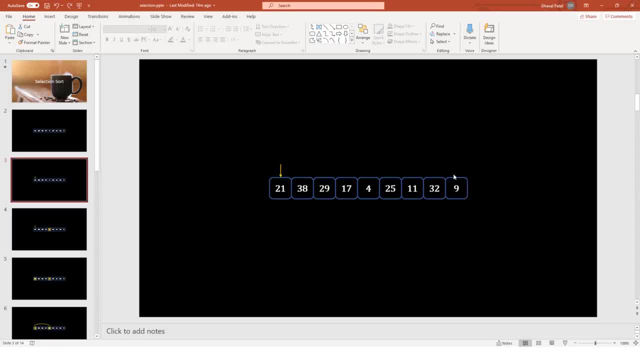 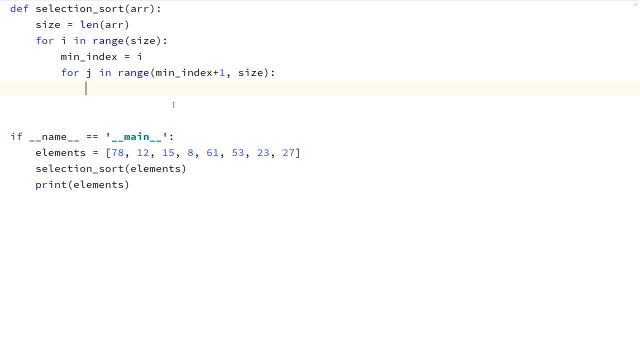 you start a loop from 38 onwards, find a minimum element and swap it with 21. so here I will say: if array of J, which means the current element, if it is less than the min index element, which is array of min index, so you have min index. if this is less than that, then my min index will become J. 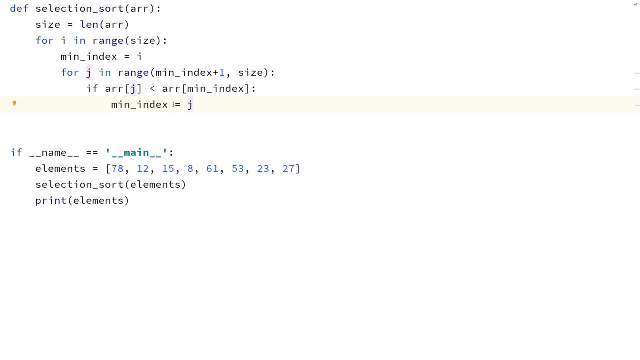 and this is equal to functions good. I hope this is clear. it's very simple. you're going through element one by one and if the current element is less than the minimum element, you're swapping the index so that now min index contains the index of the minimum element. once this for loop is over at 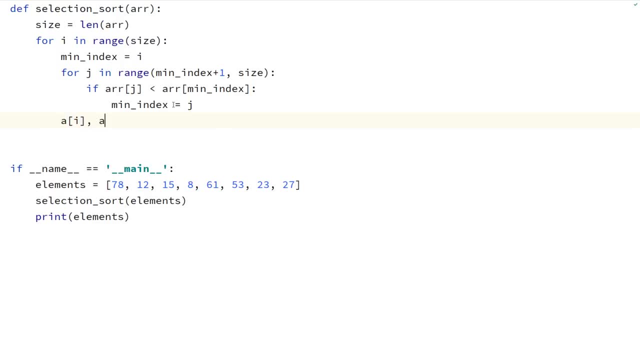 this point you are ready to swap both the elements. so you want to swap a of I with a of min index Python. this swapping can be done in one line. most of the programming language. you have to do it in three lines where you store the element into. 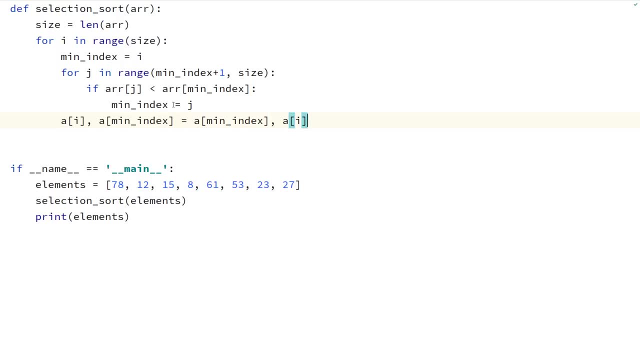 temporary element, etc. but here you can do this in one line. now we can optimize this little bit by saying that if i is not equal to min index, you know, if your is element all already contains minimum element. you don't want to swap it. this is a small improvement in terms of performance. once this is done, let's see. 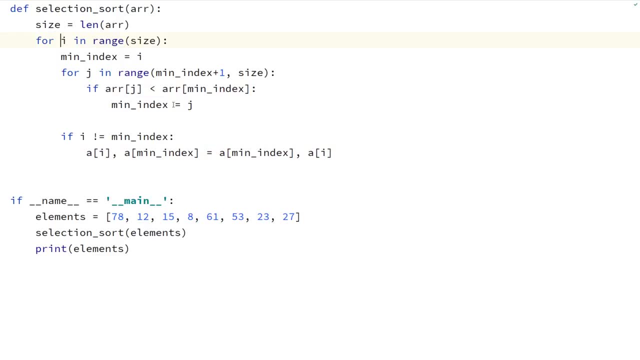 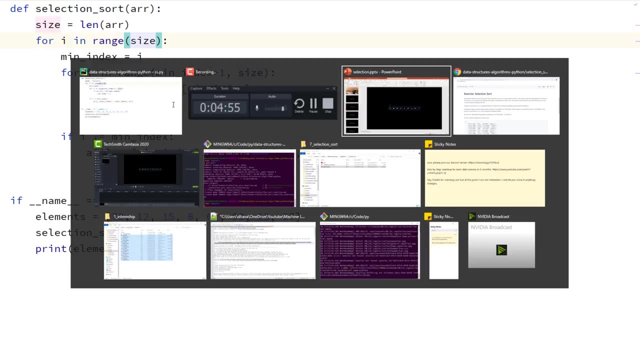 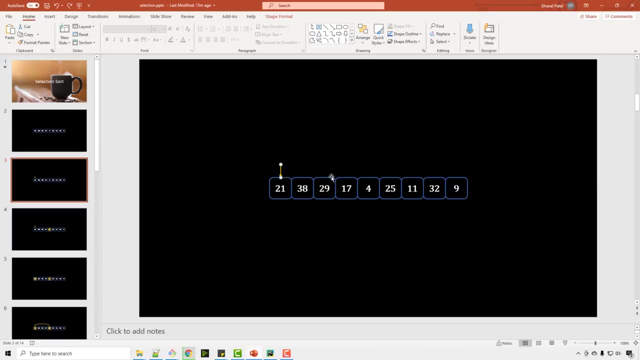 if there is any other performance improvement we can make, yeah. so see, here I don't need to go all the way till the end, because when you are, see, I'm talking about this yellow pointer- yellow pointer can go all the way till here, and if the I 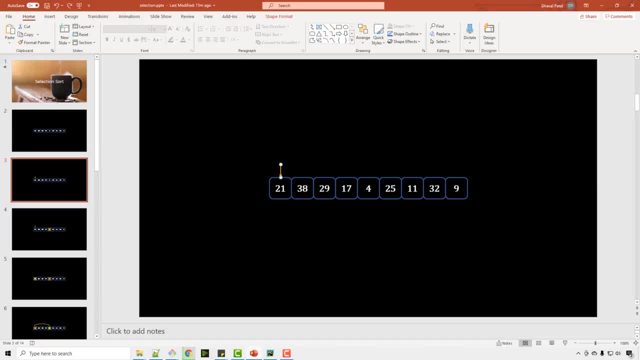 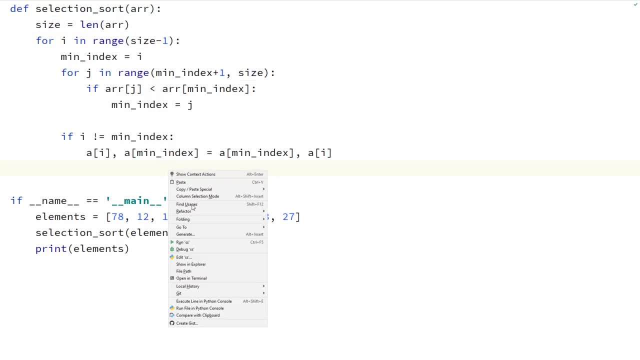 i items in this until here are sorted. it means the last element is sorted as well. so I can save one iteration here. now let's run it okay. so I will say array. there was a little typo here. you can see all the elements are now sorted. if you ever wonder how the sorting worked in,